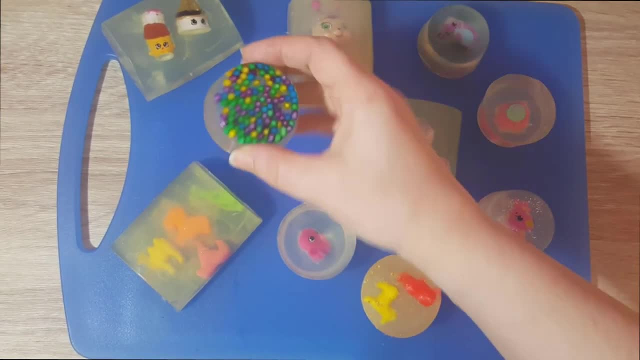 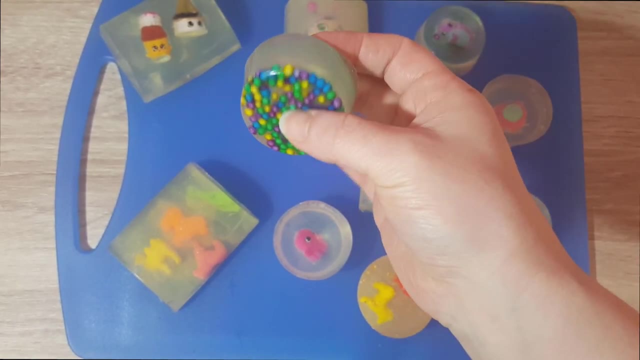 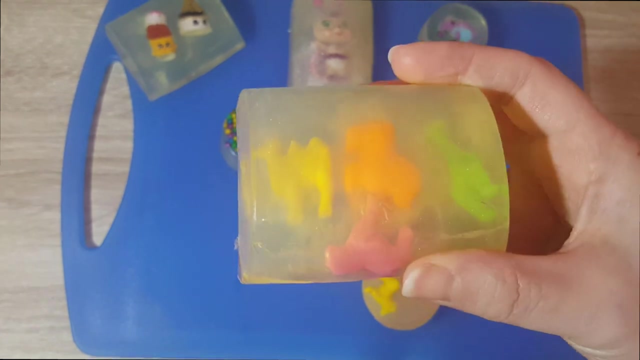 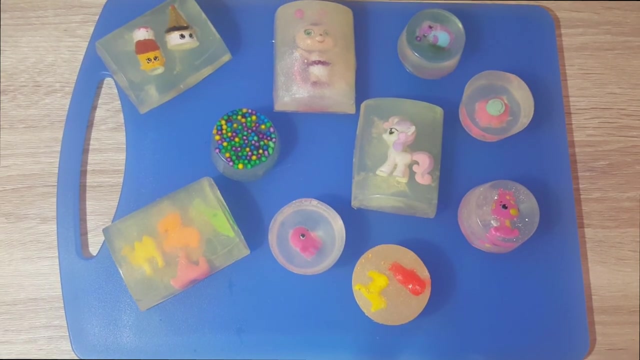 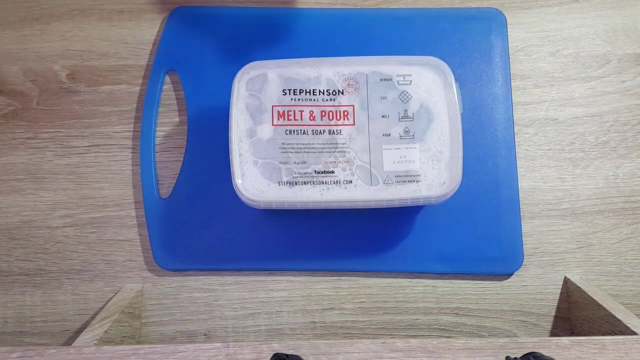 Squinkies. I've experimented with some food sprinkles and we've got some animals, So if you want to see how I make those soaps, please keep watching. You're gonna need soap base and a knife for cutting it, Spatula, wooden stick or a straw for. 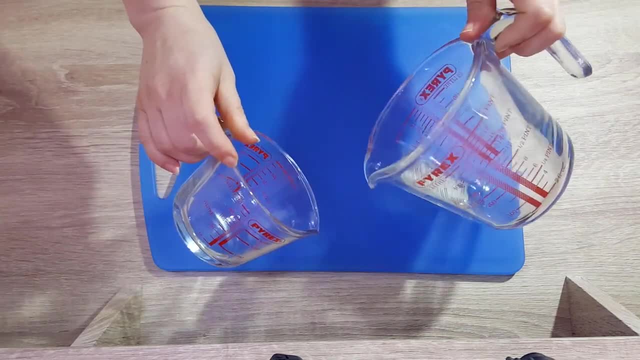 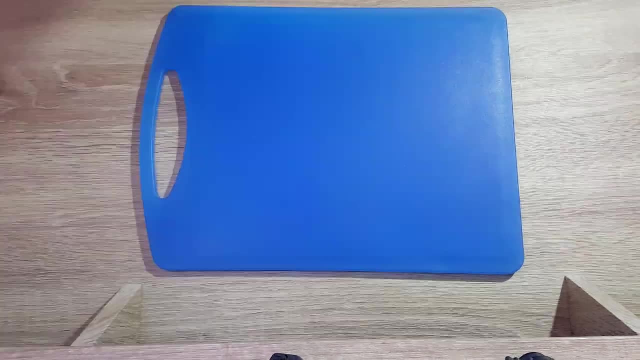 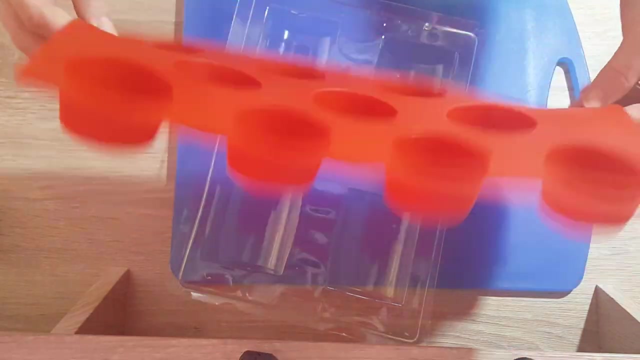 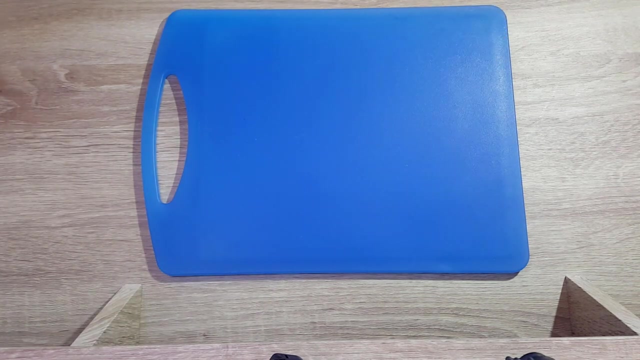 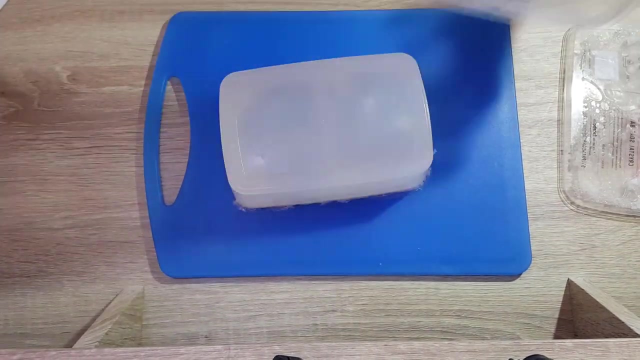 mixing Containers for melting the soap base and for dividing the portions Essential oil. I've got sweet orange here, Foot grade or cosmetic grade, glitter Soap molds and some extra silicone mold and all those small toys. I also have sprinkles angles. Let's begin. 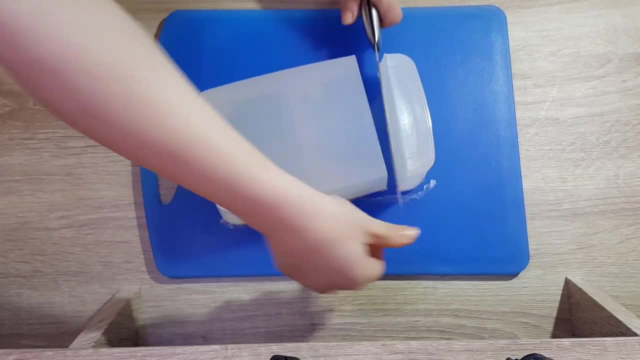 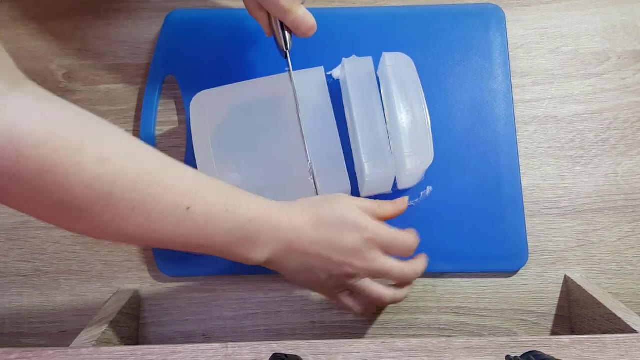 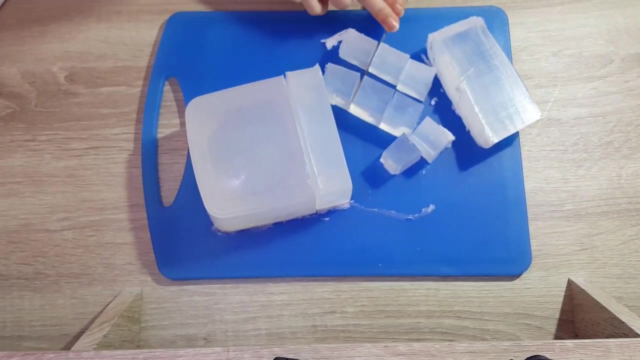 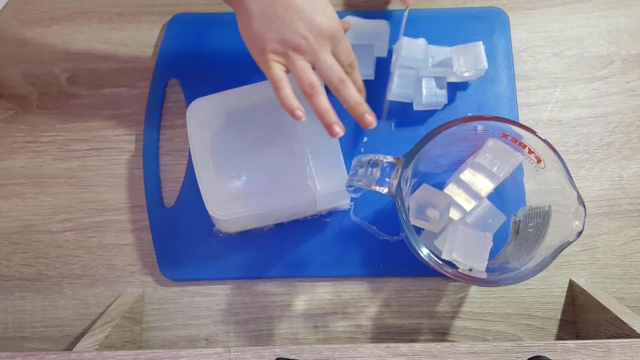 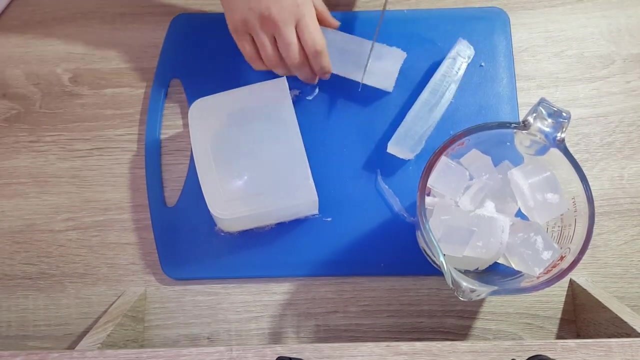 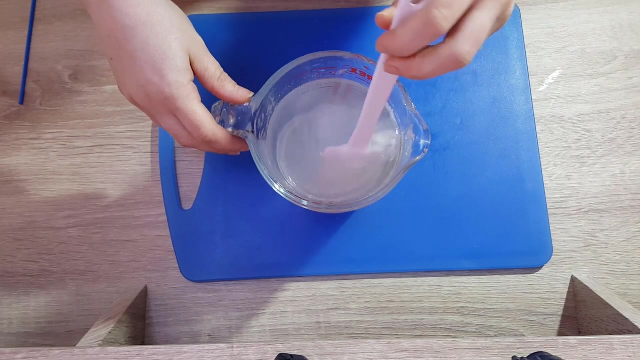 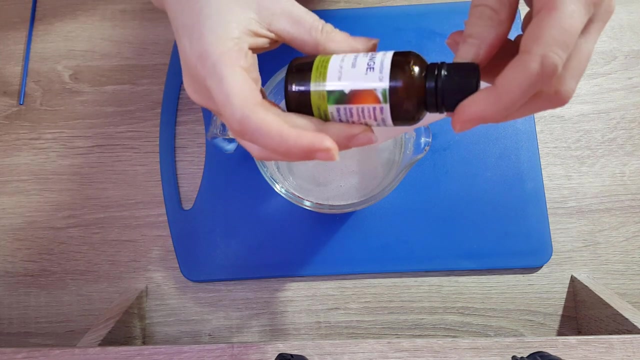 I'm going to cut the soap base into smaller cubes to make it quicker to melt in a microwave. The soap base is melted. I've had it in the microwave for maybe 3 minutes- Wow, but I was checking it throughout. Now it's time to add fragrance. 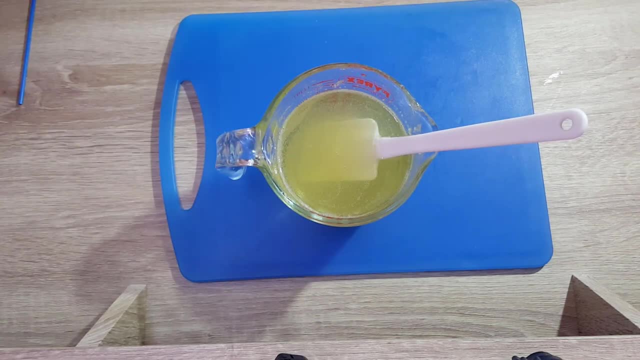 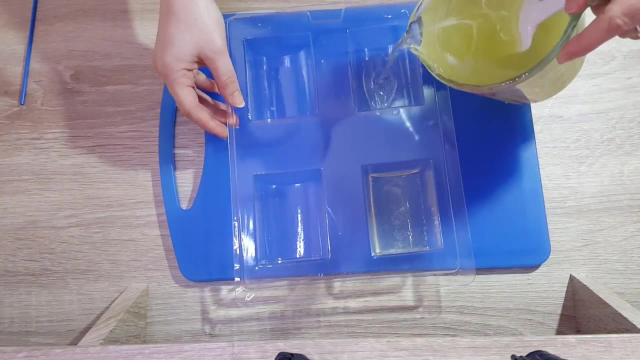 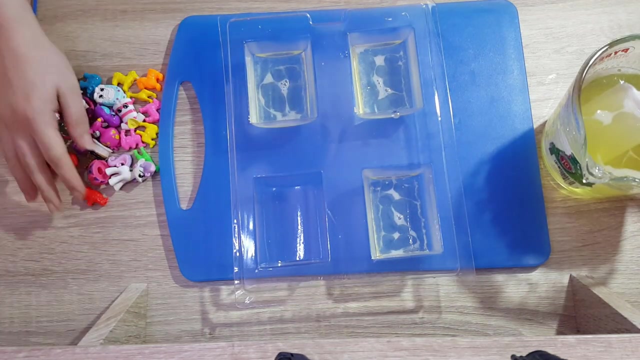 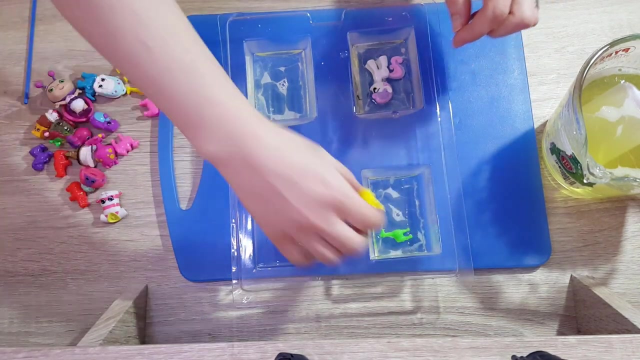 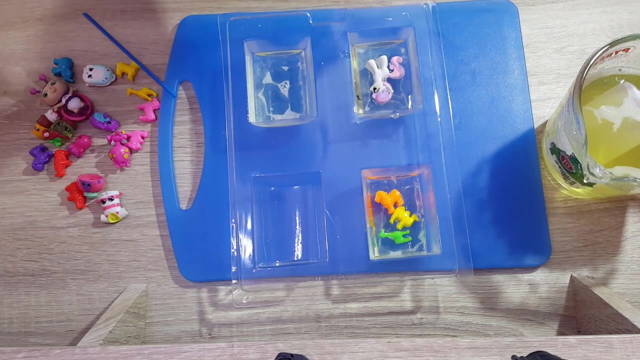 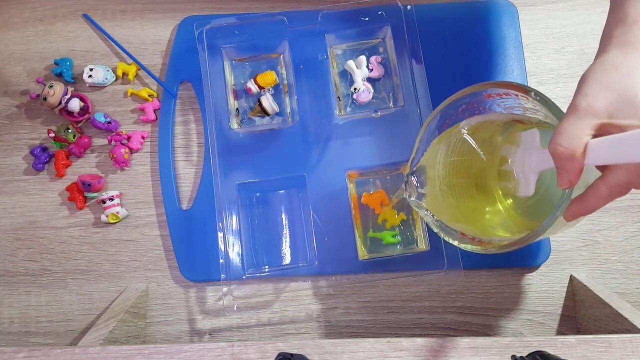 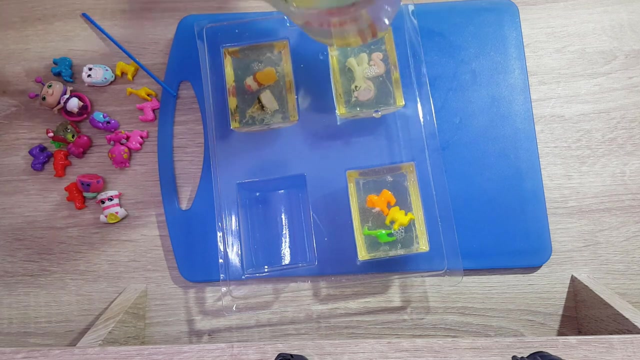 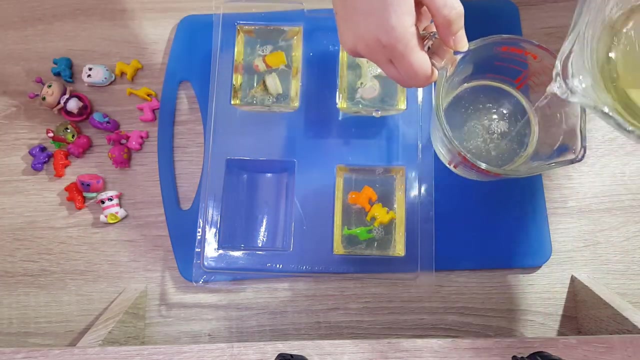 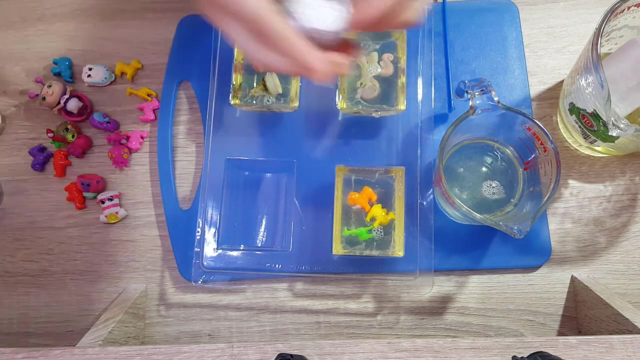 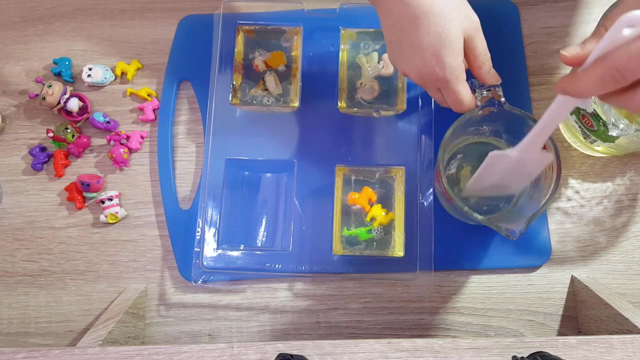 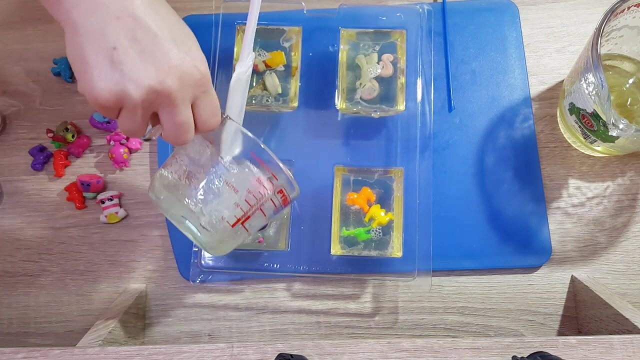 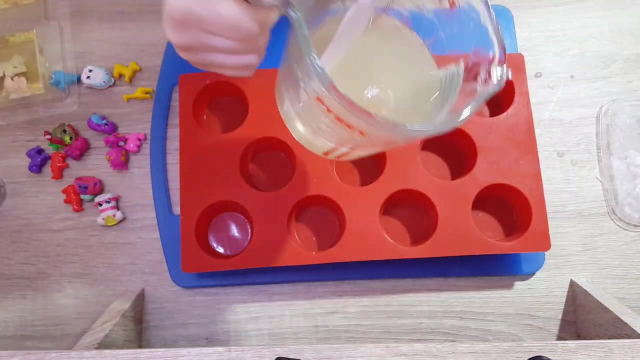 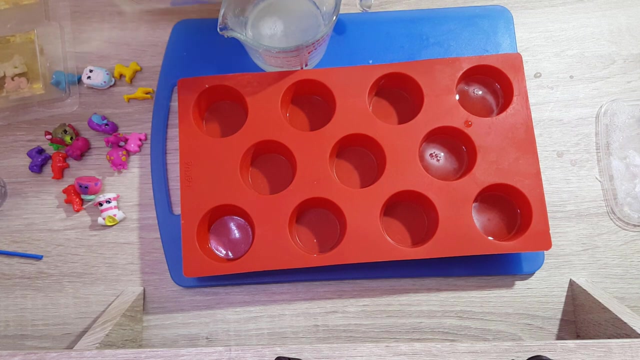 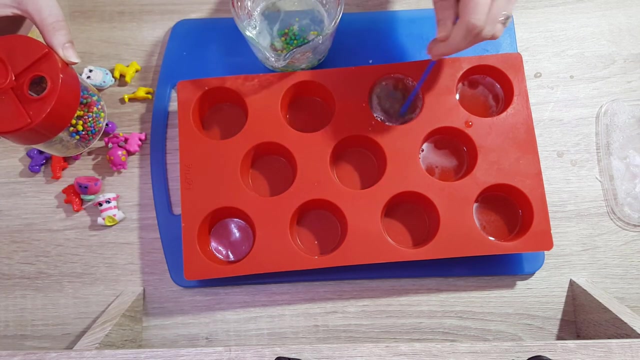 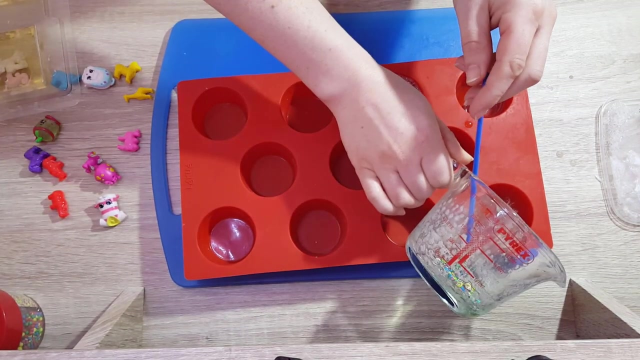 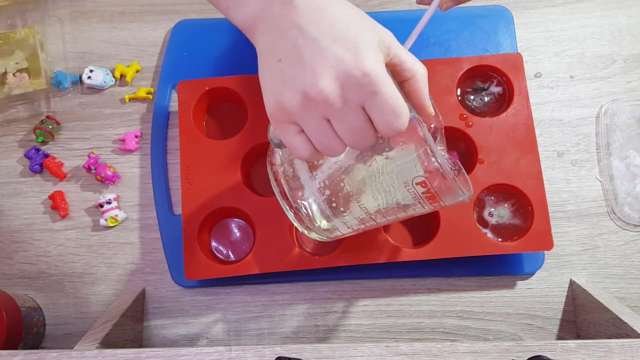 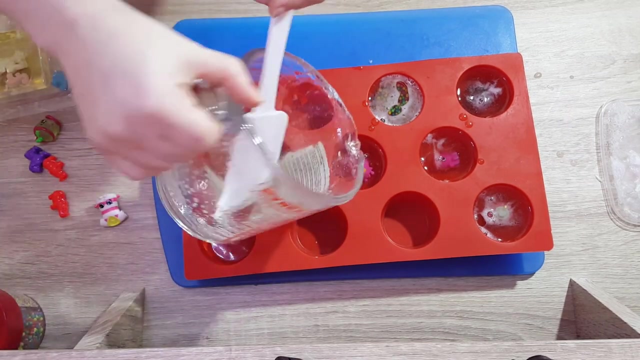 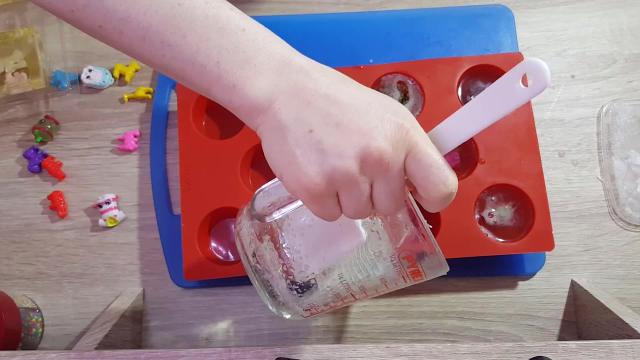 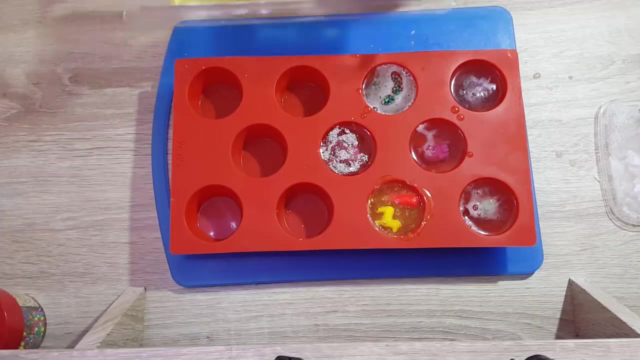 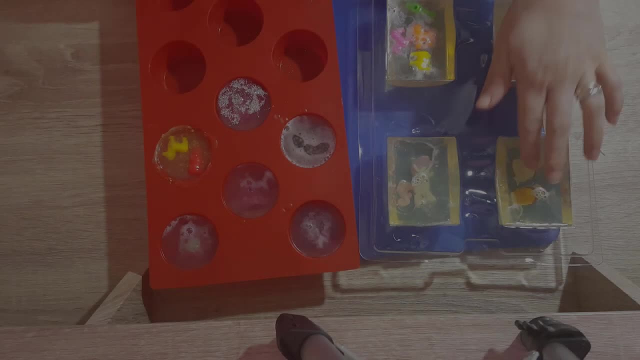 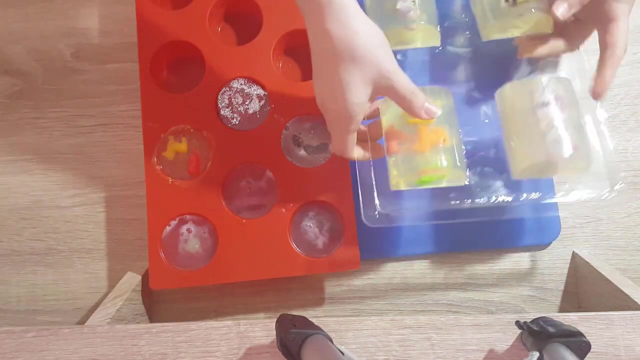 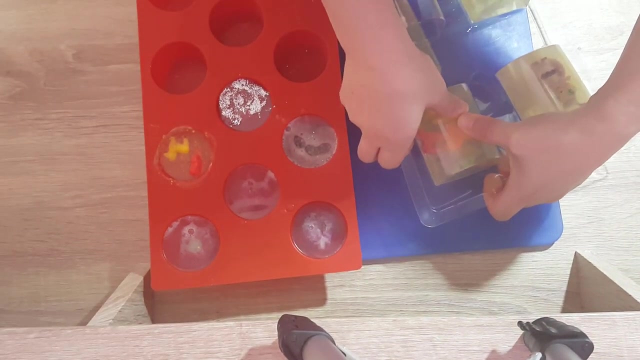 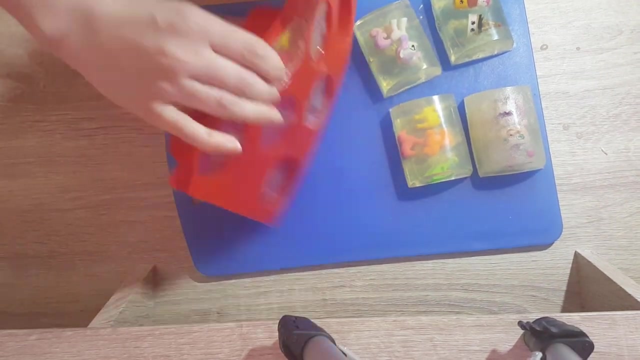 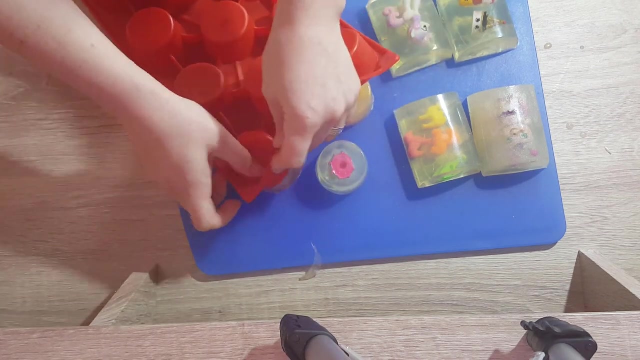 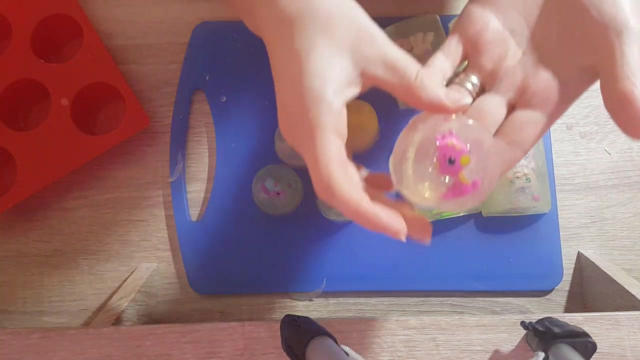 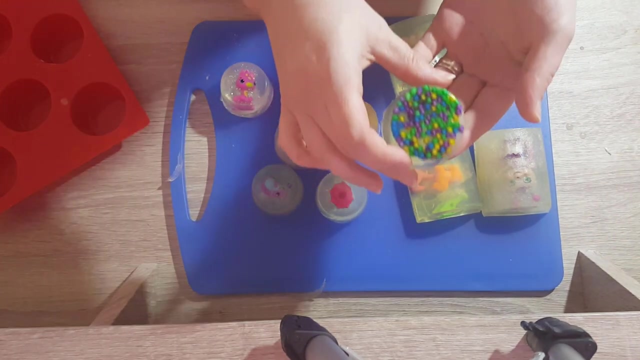